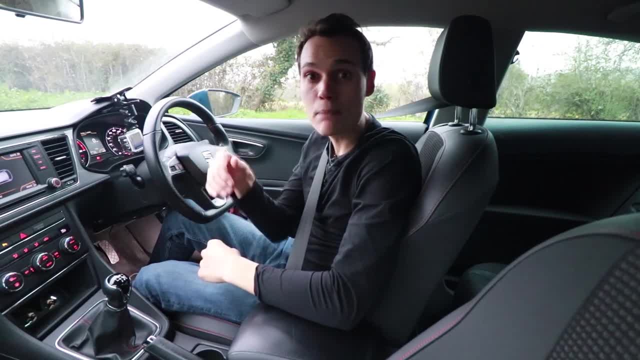 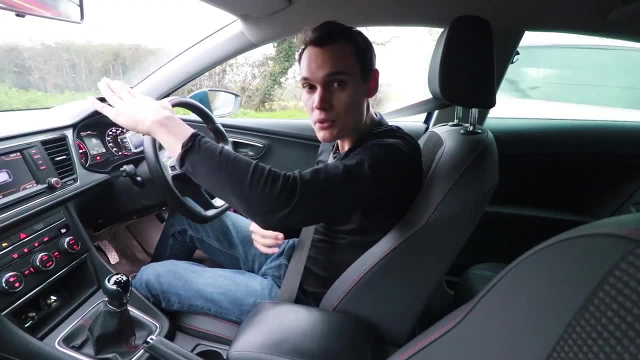 You know you're at the bite point because the engine sound goes a bit deeper, like a kind of sound. and another good way to tell that you're at the bite point is the front of your car will lift up slightly and the back will dip. On some cars you may also feel a vibration through. 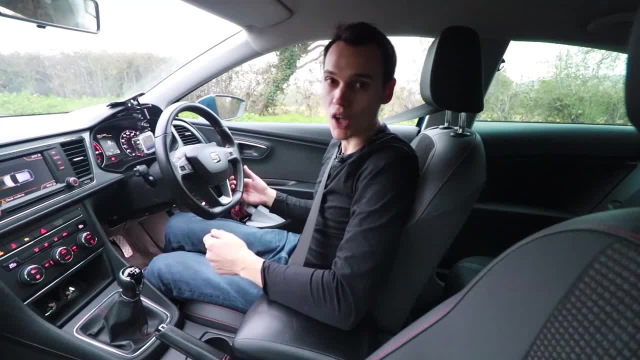 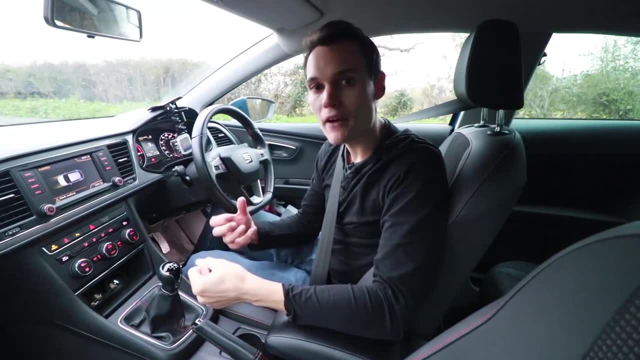 the seat and the steering wheel and the pedals, but that depends on how refined your car is. The pro of using the handbrake to do a hill start is that it works in any car- New, old, powerful powered. you'll be able to move away uphill without stalling. The downside is it takes a bit of time. 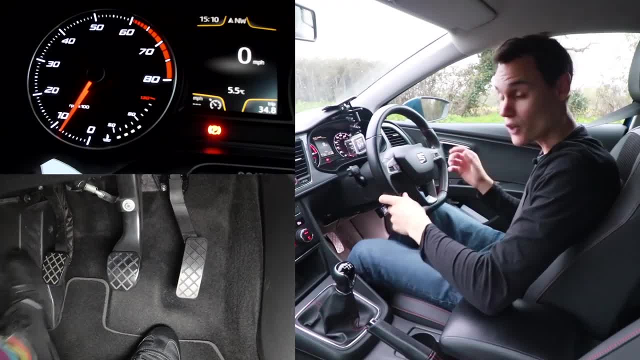 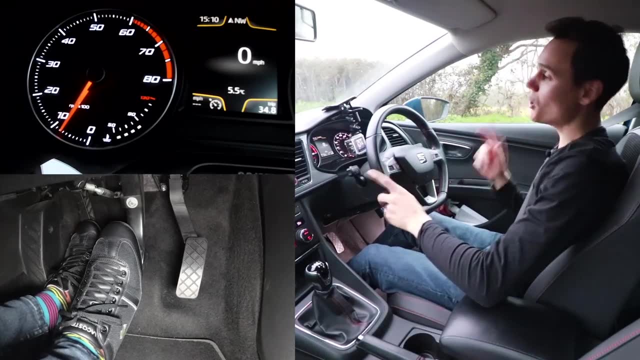 Another way is to find the bite point whilst your foot is on the foot brake. So clutch down first gear, foot on the foot brake and handbrake off. So now, if I come off the foot brake, I'm going to roll back, as you know, but if I lift the clutch up to the bite point, there it is and then check. 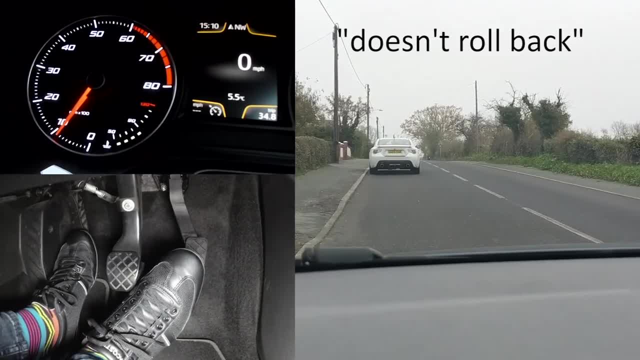 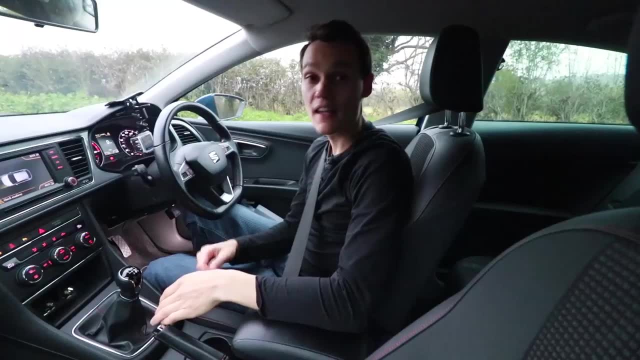 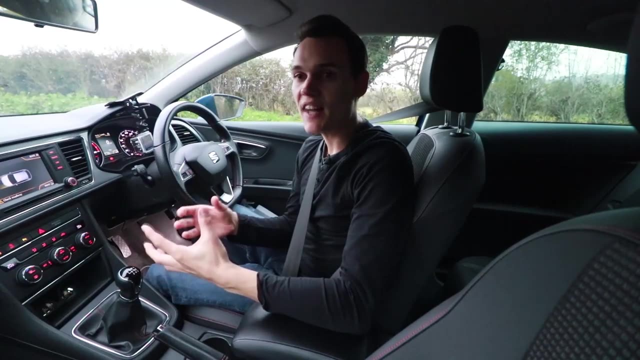 around and make sure it's safe and come off the foot brake. the car doesn't roll back. In fact, it starts rolling forwards. Add some gas and accelerate a little bit faster. the advantage of this method? well, you don't have to do much work, you don't have to pull a handbrake on and take it off. the disadvantage is that you 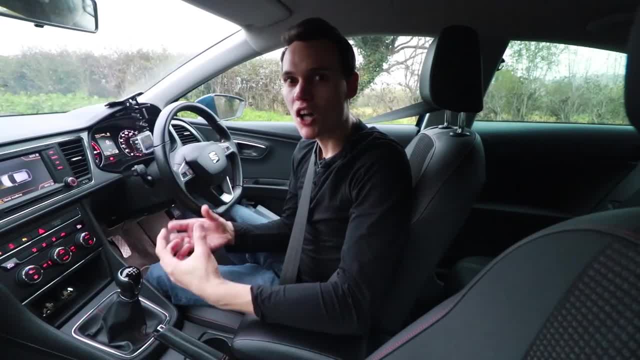 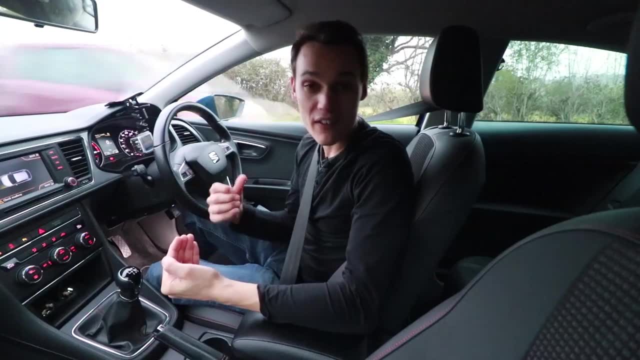 might stall. older cars certainly will probably stall and newer cars will struggle, if not stall. now it's not good to move away with the car struggling. if you lift the clutch up to the bike point without gas in a new car it will stop itself from stalling, but it's not going to have. 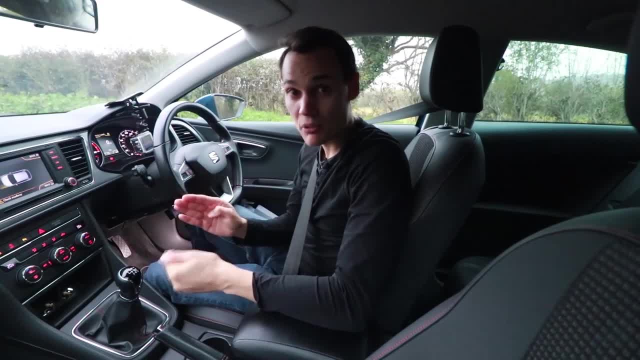 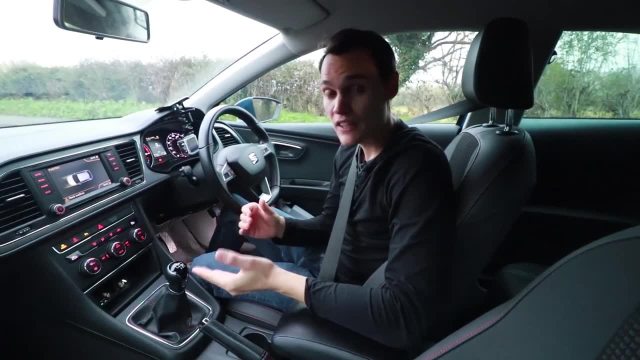 much power and it's going to vibrate quite a bit if you use the gas and bring the clutch up the bike point. without gas to the bike point, the car's going to move away a lot more cleanly and smoothly. having said that, if you know your car well and you know that you can lift the clutch to the bike point without it, 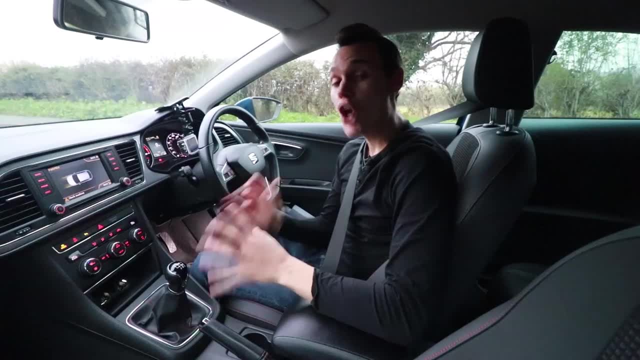 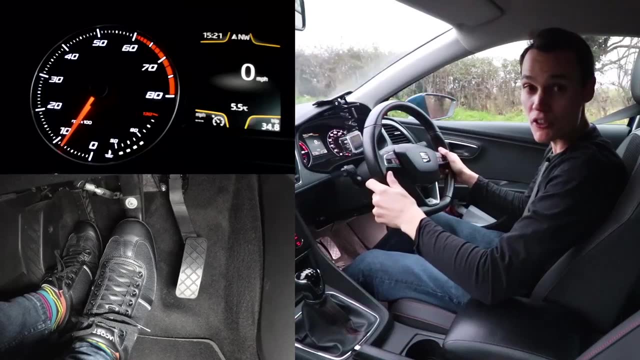 struggling or stalling. there's not much wrong with doing that method. but if you're learning to drive, you want to learn a method that's going to work in all cars, not just a certain percentage of cars. another method is to try and do it really quickly. so come off the brake, press the gas and lift the. 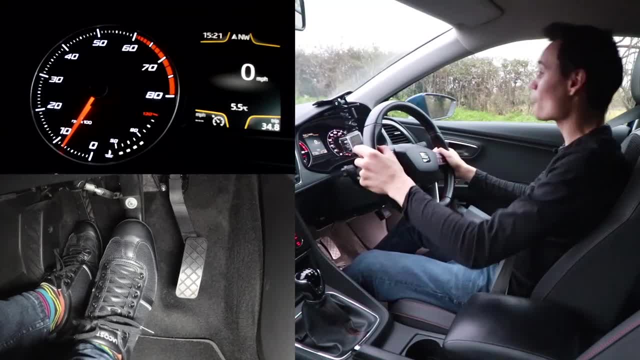 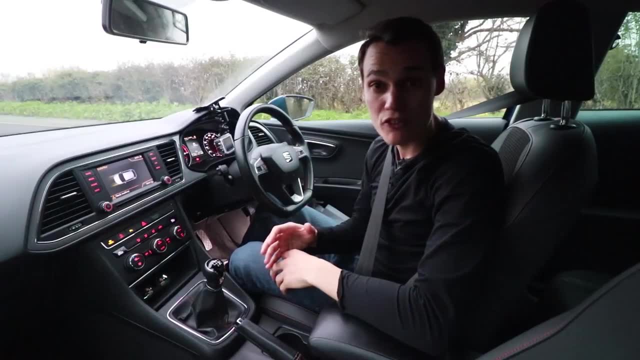 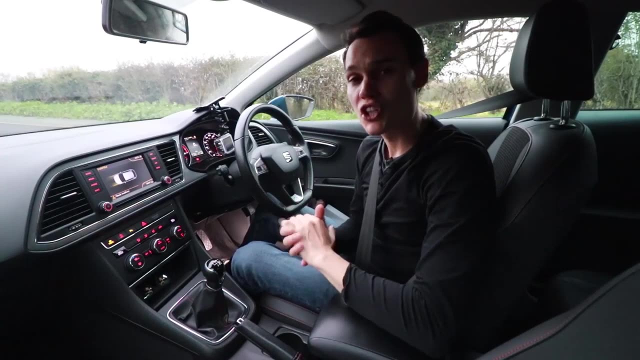 clutch up quickly and hope you don't roll back. so now i'm coming off the brake on the gas, lift the clutch up, roll back a tiny bit, but it worked. the pros of that method: it's quick and easy. the cons of that method: probably impossible if you're a learner driver. what a learner is likely to do in? 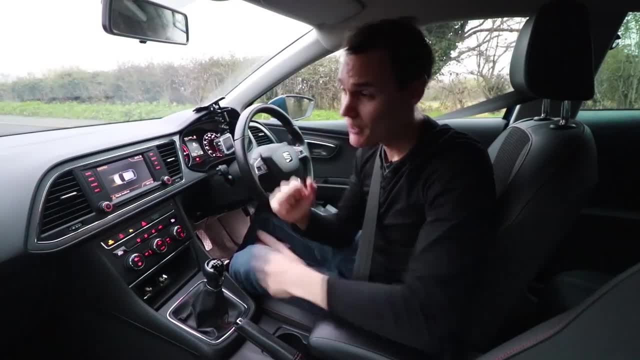 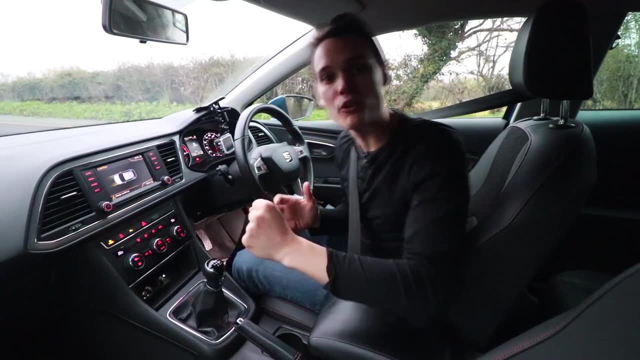 that situation is: press the gas way too hard, give way too many revs, bring the clutch to the bike point, burning it out in the process, rolling back in the process or shooting forwards or kangarooing up the road. if you're learning to drive and you try and do that method, you're probably going to 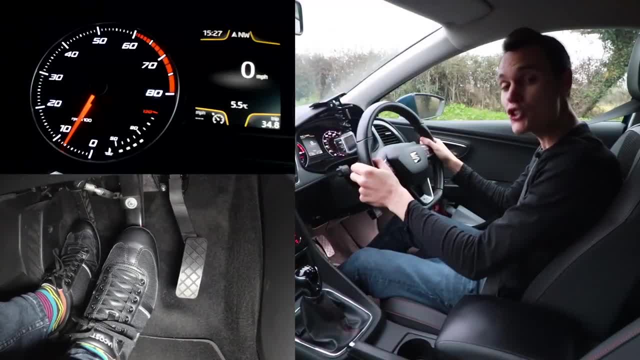 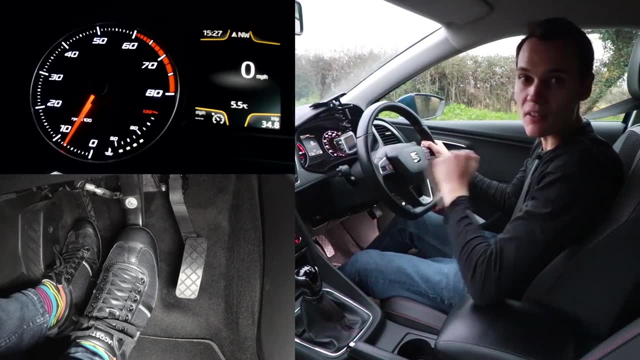 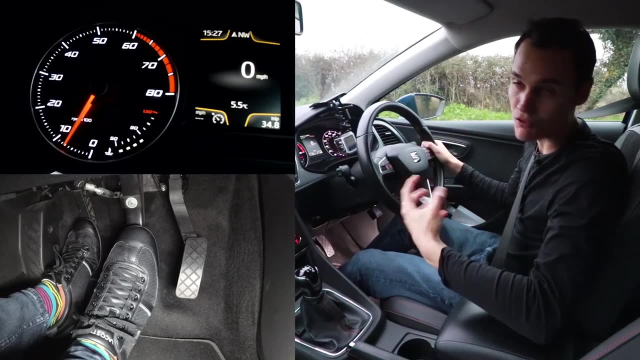 learn to hate driving pretty quickly. another method is to use hill hold assist. not all cars have this, but if yours does, it can make moving away uphill a bit easier. what it does is when you come off the foot brake to go to the gas is it stops you from rolling back. it holds the brake for a couple of seconds, for example. 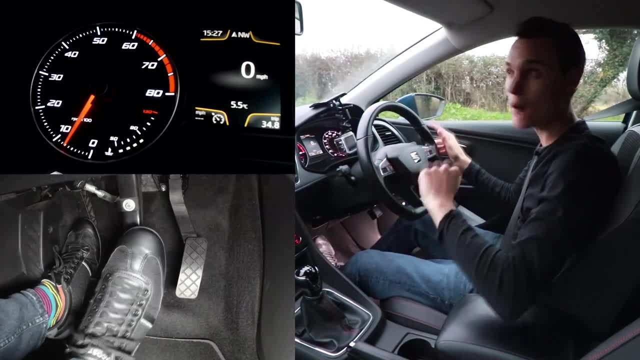 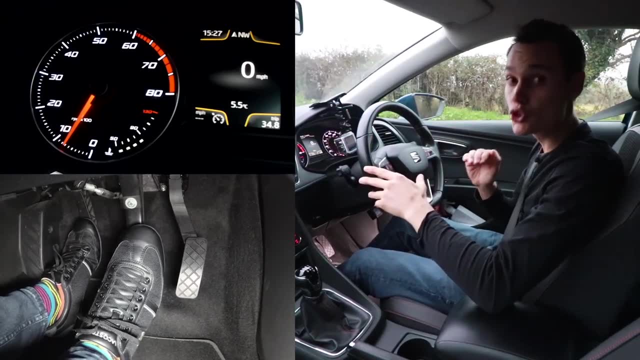 when i come off the foot brake. now i'm off and the car's not moving. now it's rolling back. that should give me enough time to get my gas and clutch ready. the moment you press the gas, though, the brakes do release, so it's still a very 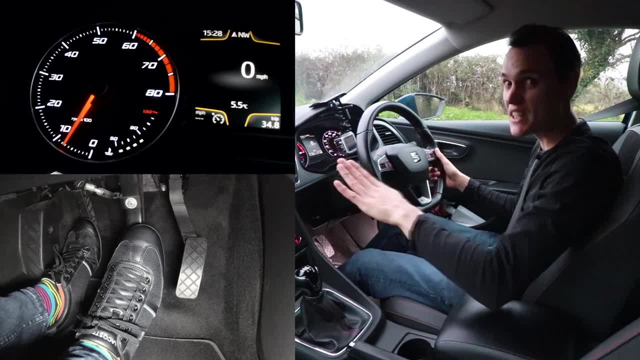 tricky method to do. but if you're learning to drive and you're learning to drive and you're learning to do, but if you're learning to drive and you're learning to drive and you're learning- tricky method for learners, as you do have to bring the clutch up to near the bike point and then 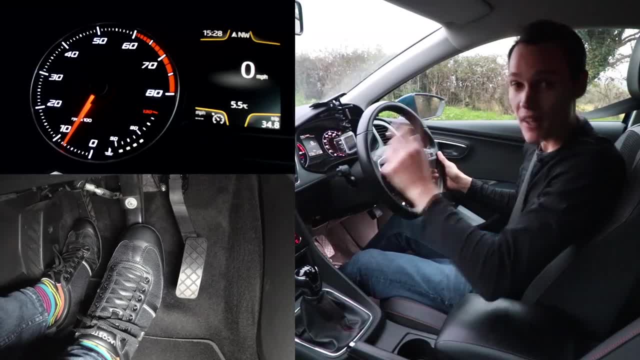 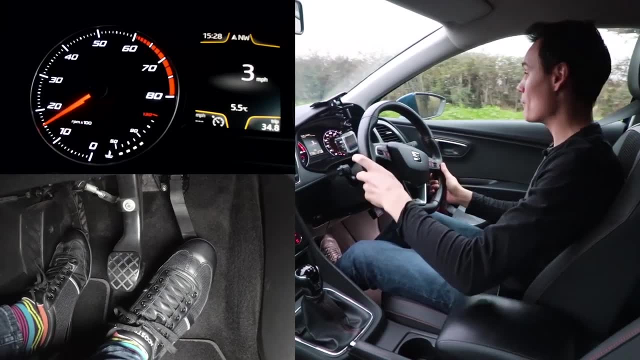 press the gas and lift the clutch the rest of the way. that's kind of how you do it, let me show you. so no one's coming, i come off the brake, get near the clutch bike point, add the gas and lift the clutch. the bike point a little bit more and i'm away. quite easy for me, because i know exactly. 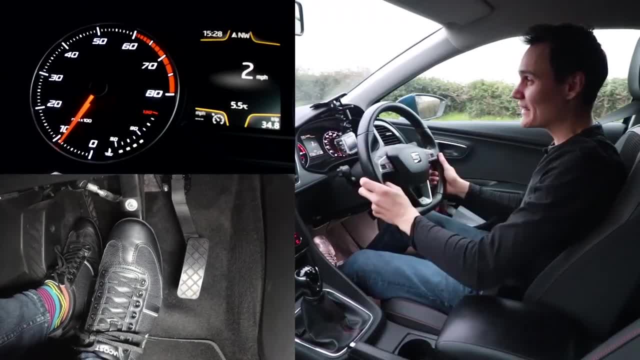 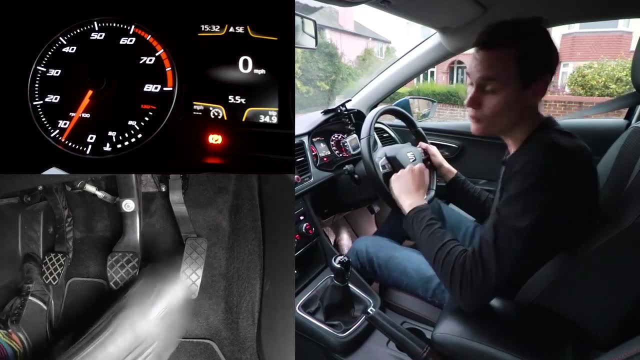 where my bike point is. but again, for a new driver that method is quite hard and not all cars have it. now for some downhill starts, the first one handbrake start downhill, so clutch down first gear handbrakes on, get some gas, find the bike point. 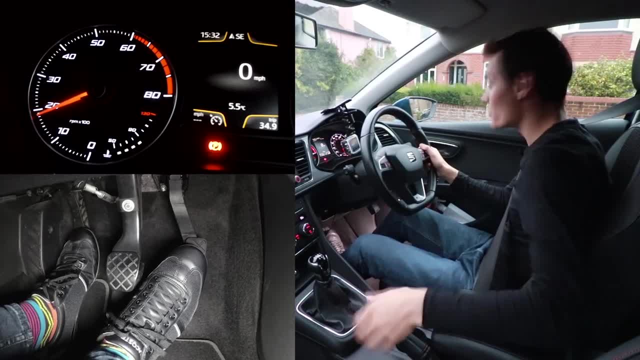 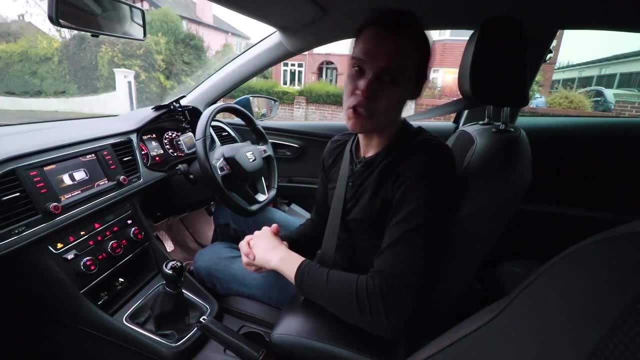 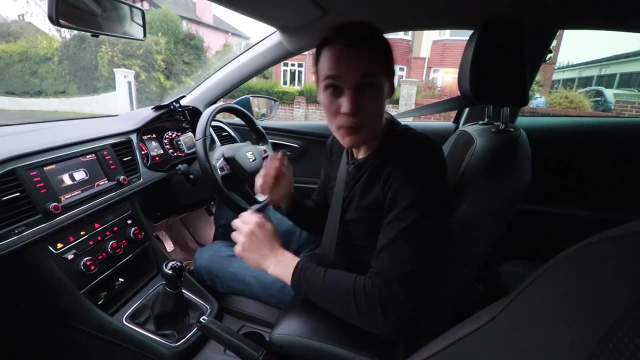 there it is and then make sure it's safe to go and handbrake off and i'm going. this isn't really a very good method, if i'm honest with you. i can't think of many pros. maybe one if you are very inexperienced at driving and it takes you a long time to get your gas and clutch ready. you could. 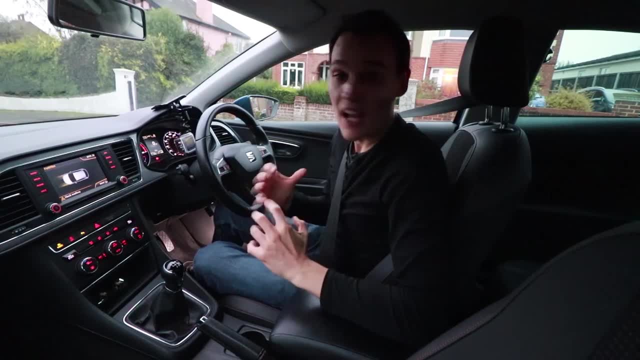 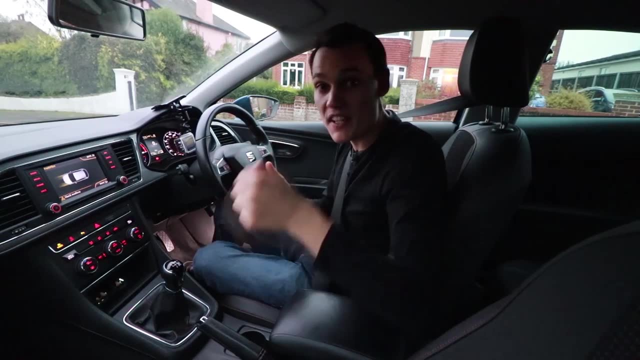 have the handbrake on when you're at a junction downhill and whilst the car's going to be in past, you can get your gas and clutch bike point ready to go so that when the last car passes you take your handbrake off and you move immediately. but you don't really need to do that because 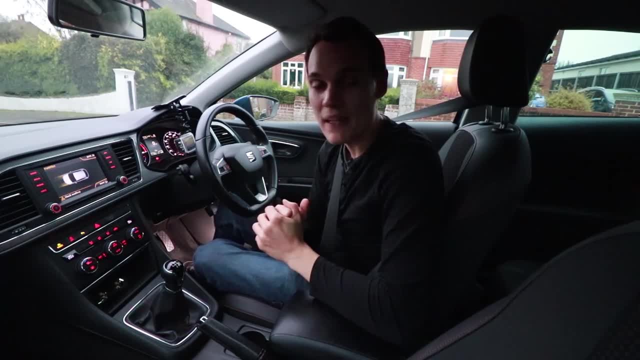 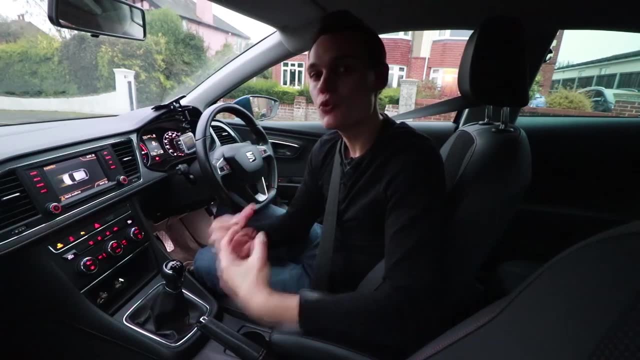 downhill. when you come off the foot brake, the car rolls for you anyway. so i recommend just coming off the foot brake downhill and get your gas and clutch up as the car rolls and use the hill to help you. part of driving a manual car is to put the hill to work, is to get it to slow you down. 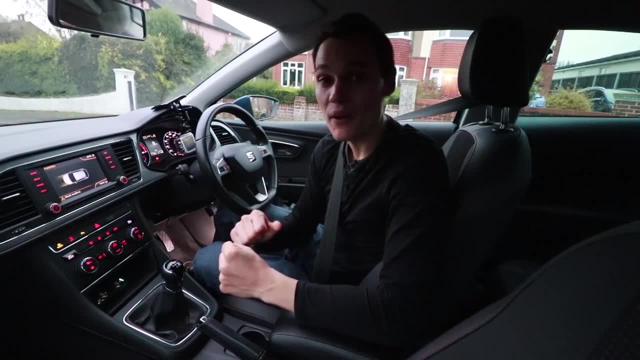 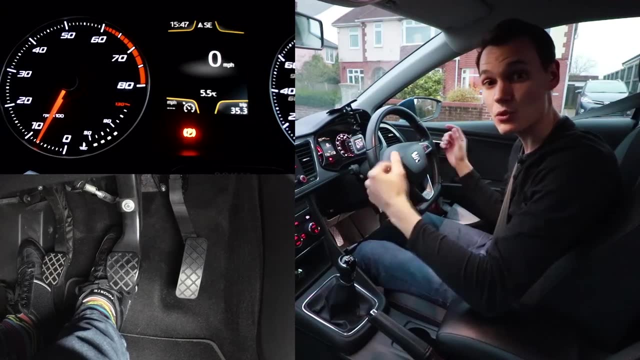 when you're going uphill, and it's to get you to get it to work and it's to get you to slow you down, it's to speed you up when you're going downhill. another method for moving away downhill, which is my preferred method and the most normal method, is to get the hill to start you. let me show you. 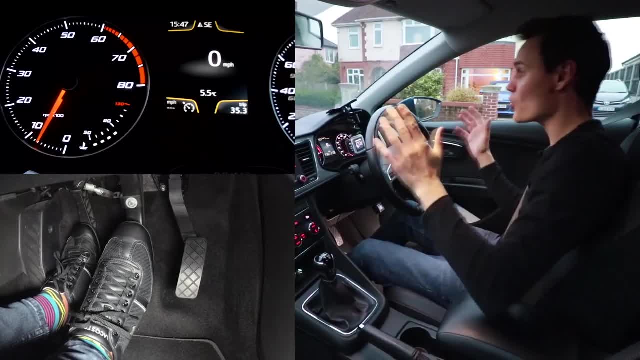 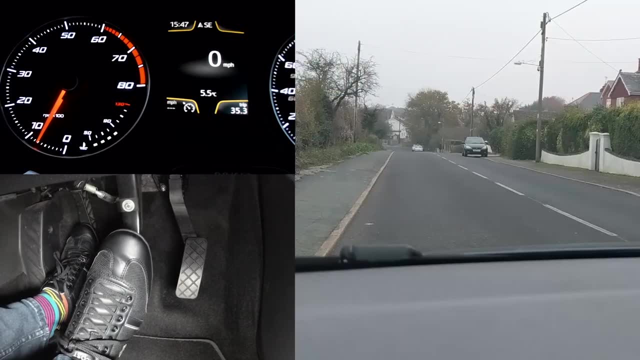 guys now first gear, foot on the brake and handbrake off the hill wants the car to roll forwards. now, that's handy, let's put it to work so no one's coming. come off the foot brake and the car starts rolling. and what's great about this method is that how fast i roll is down to me if i. 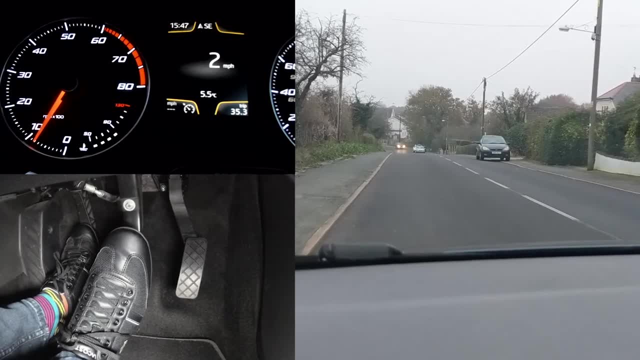 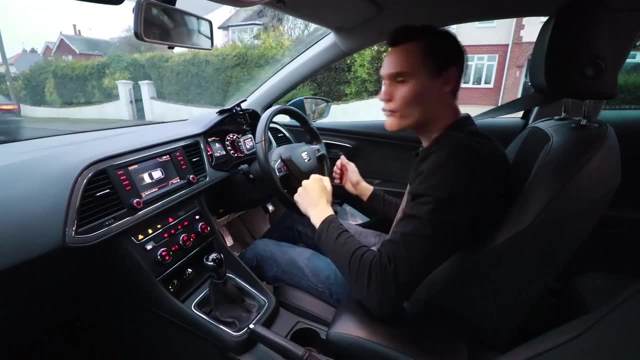 use the brake now i can keep myself slow. if i come off the brake, i can keep myself slow. i will speed up. there's a break again to slow down. i'm just going to stop now, and what's great about that is that if there's a car in front of me, i can stay really slow and drive around it without 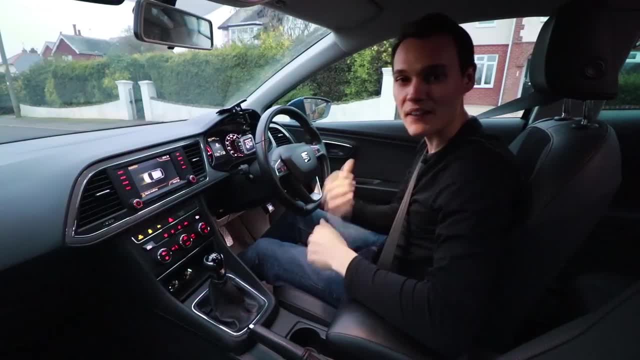 shooting forwards. however, you can't keep the clutch down the whole way down the hill. you will need to bring the clutch up once you reach about five miles an hour to avoid coasting where you lose engine braking. but that is another video. another method is to move away in second gear. 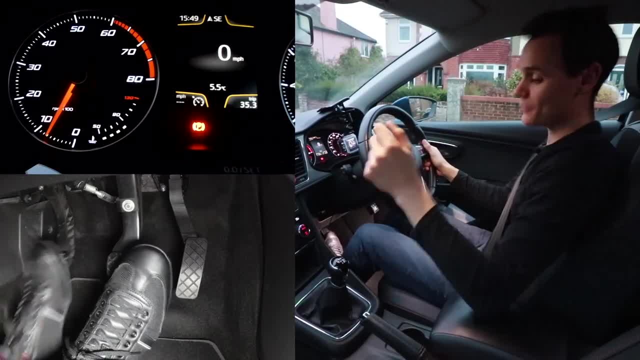 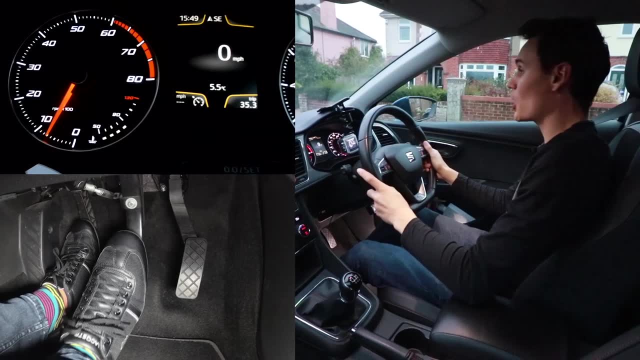 when you're downhill, instead of first gear, that can actually be quite handy. so clutch down into second foot on the foot brake and handbrake off, and when no one's coming i'll come off the foot brake. a little bit of gas, a little bit of bite point in second gear. 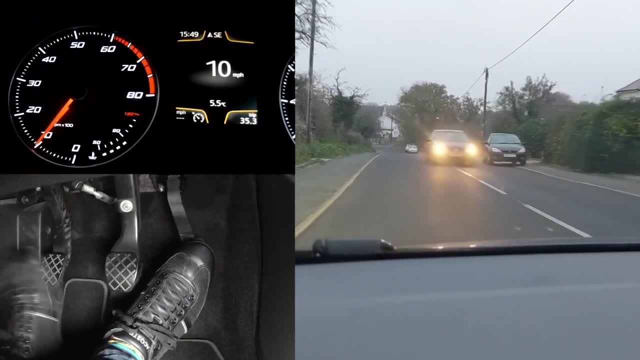 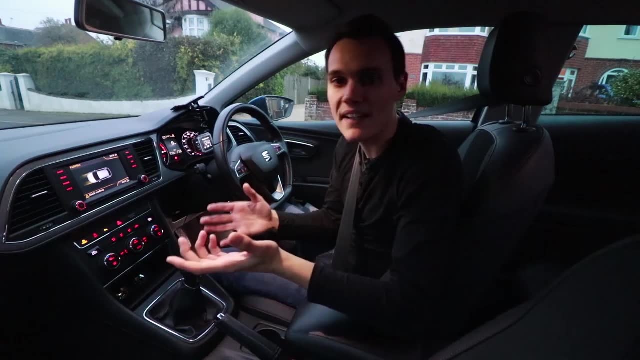 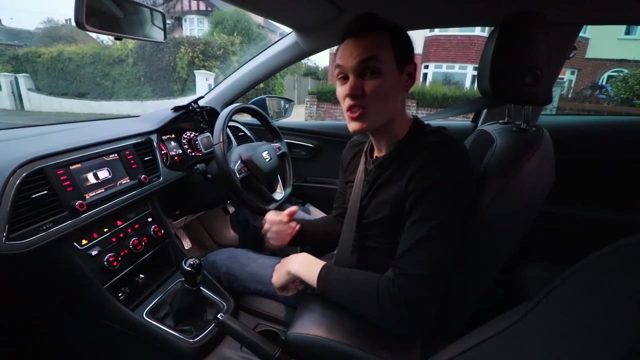 hold the clutch for a second or two and then come off the clutch and now i'm moving. why use second gear then? why not use first? why make it complicated? well, it makes it a bit easier, actually, because if you start in second gear, you're not going to have to change the second gear later, so you're. 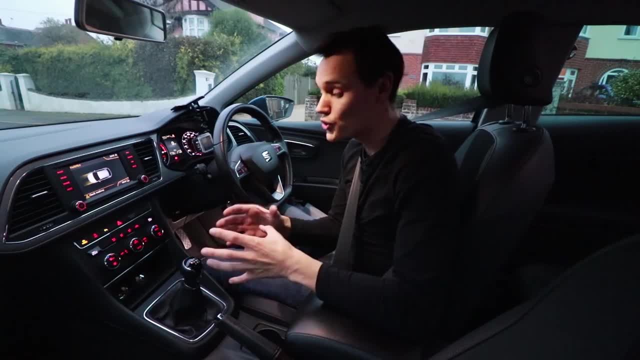 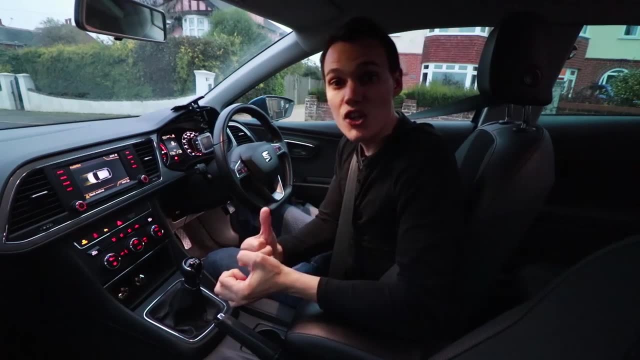 saving yourself a gear change, and the reason why you can use second gear downhill is because the hill is adding power for you. the hill is helping you move forwards, so you don't need the extra pulling power of first. and remember: low gears have more power. you don't need the extra power.